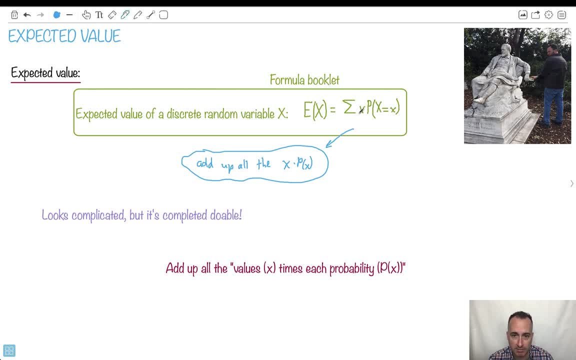 But basically, you take every x, you multiply it by the probability, you multiply it by the probability of getting that x and you just add up all those. So if you had three different situations, then you've got to do, you know. 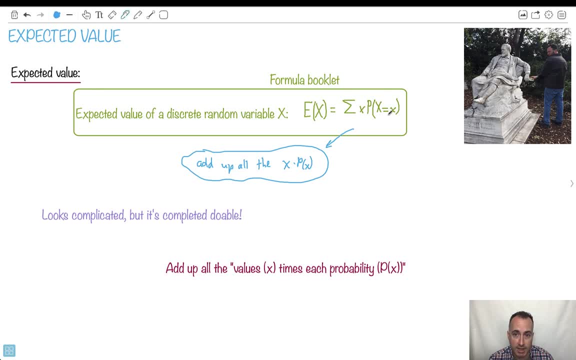 the first one times its own probability, plus the second one times that probability, plus the third one times that probability, and so on. So although this looks complicated, it doesn't have to be So. let me show you. I've got a few different tips to give you. 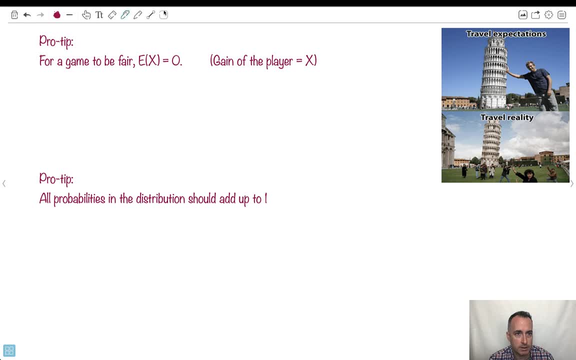 If something's going to be a fair game, it just means that the expectation, the expected value, is going to be zero. So that's the gain of your player. So we expect that to be zero. This one here. look at this. 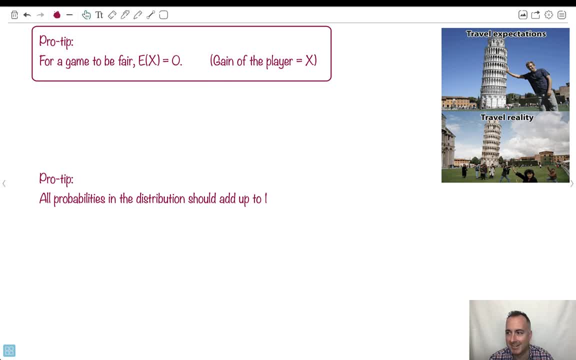 So travel expectations, travel reality. That was kind of cute actually. Also, we know that all the probabilities right here, actually you know what I'll do. I'll remove the gain of the player part actually, because that's not quite. 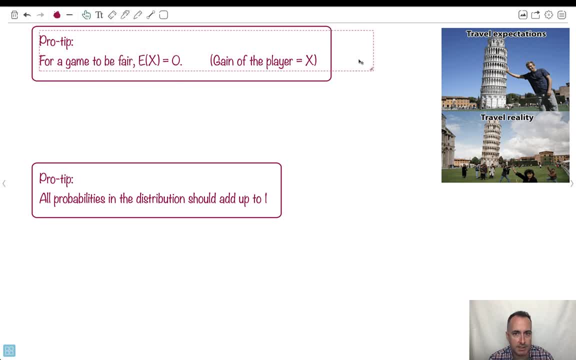 it depends how you look at it. It could actually be misleading, I think. Let me just change the text here and I'll just I'll remove the gain of the player part. That's maybe not. I'm worried that it might be a little bit misleading. 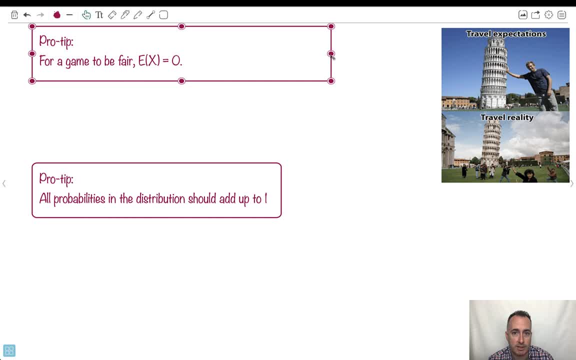 The expected value is zero. I think that's the better way to say it. There you go, Changed my mind. There we go. So for a game to be fair, expected value is zero. In other words, the player shouldn't gain anything, or at least the expected value should be zero. 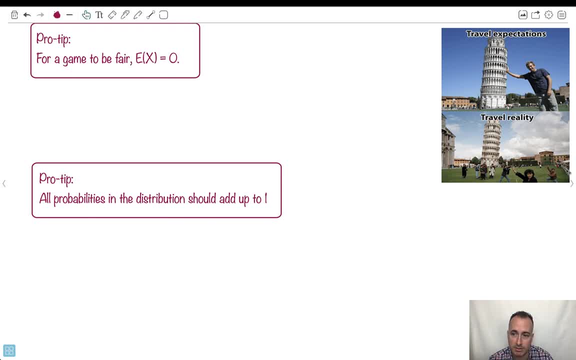 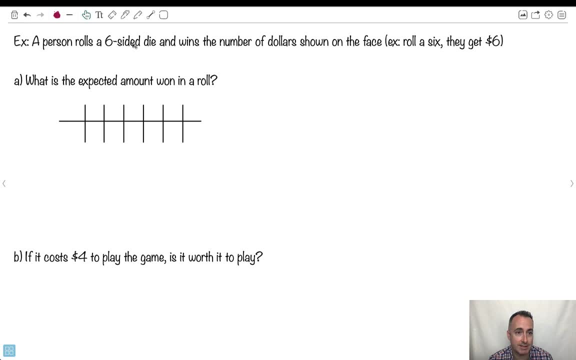 Probabilities should all add up to one. as usual for probabilities, This one just makes me laugh, And let's go ahead and do an example. So a person rolls a six-sided And you win the number of dollars shown on the face. 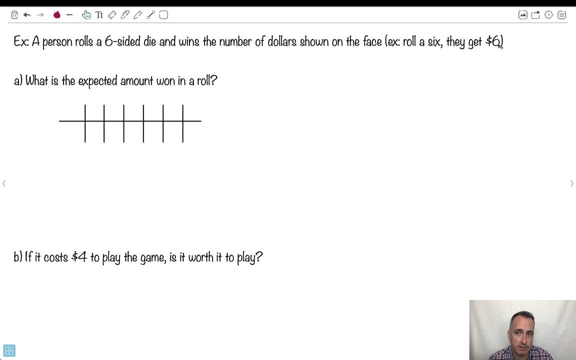 So, for example, if you roll a six, you get six dollars, If you get a- I was about to say- seven, If you get a three, you get three dollars, and so on. What is the expected amount won on a roll? 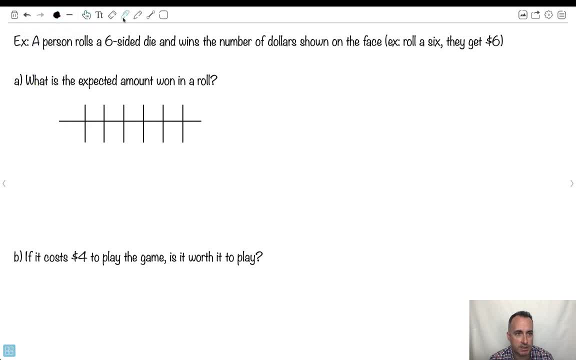 So what I'm going to do, I'm going to show you how to set up this thing with these discrete, random variables. So I'm going to say lowercase x, a little x, and we might have different outcomes. We might get a one or a two or a three, or a four or a five. 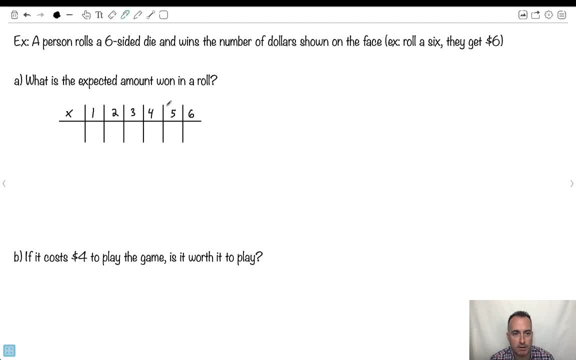 Or a six. Now we're going to assume it's a fair die. In other words, the probabilities of getting each of these will be the same. But watch carefully. I'm going to say the probability of my discrete, random variable capital X being lowercase x. 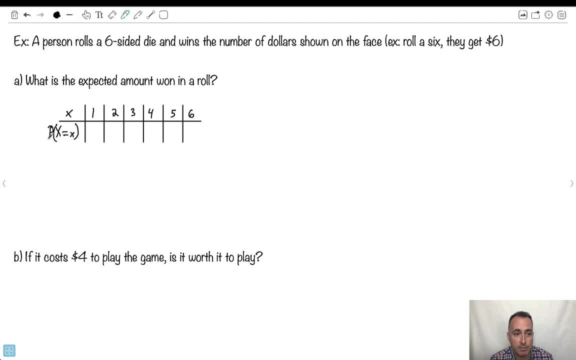 I'm just using the proper notation here. What it really means is: what's the probability of getting a one? Well, it should be one over six. Does that make sense? The probability of getting two should also be one over six. This should be one over six. 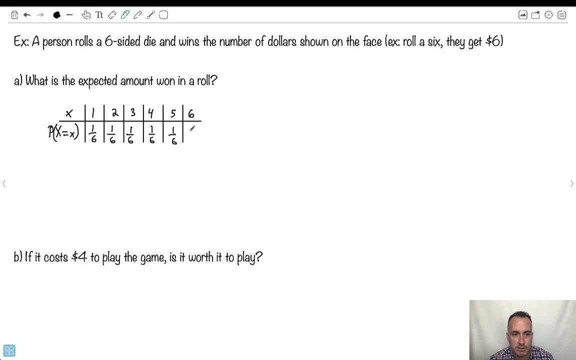 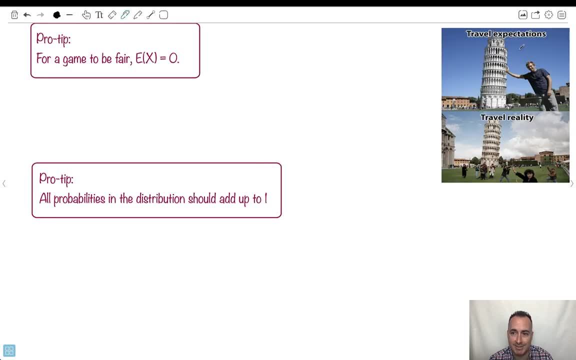 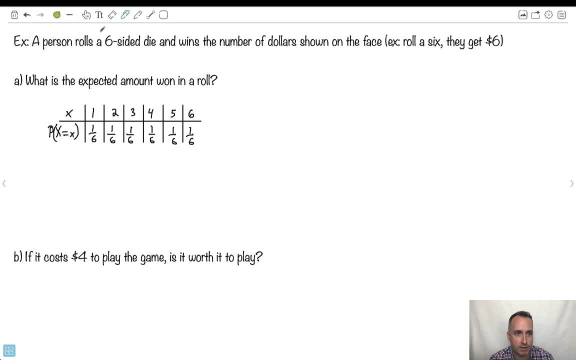 All right, So let's do the expected value now. So I'm just going to write down the formal equation for expected value. It's just going to be the sum of all the x's times all the p of. I'm just going to write lowercase x, just like that. 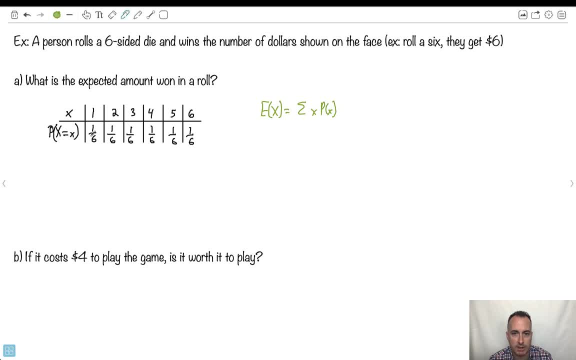 I'm not going to bother with capital X equaling lowercase x. I'm just going to be a little bit sloppy and just go add up all the x's times, the p of x's. Well, watch carefully, then I know all these values. 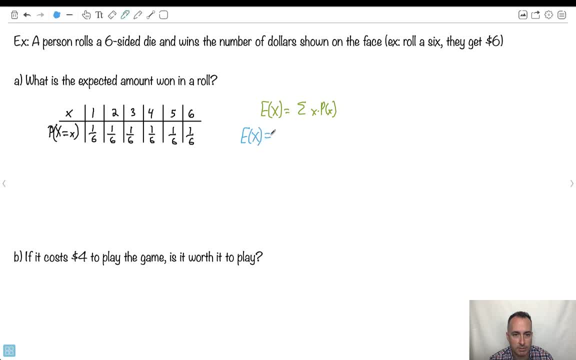 Look the expected value, then capital X. here is going to be: let's see, one times one over six, Do you see what I'm doing? Plus, let's see the next one. So two times one over six. 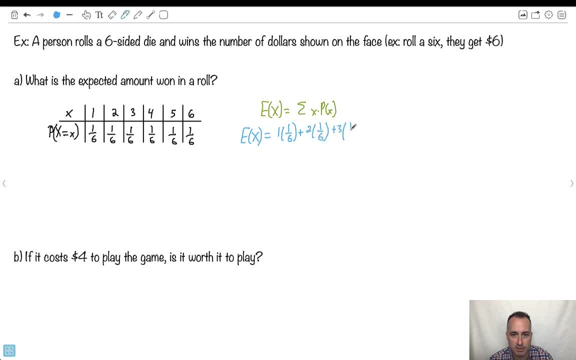 Now, sometimes these are different, so you have to be very careful. In this case, it's going to be pretty easy. It's just keep going like this, right? I just add up each of the x's times its probability, so the probability of getting that x value. 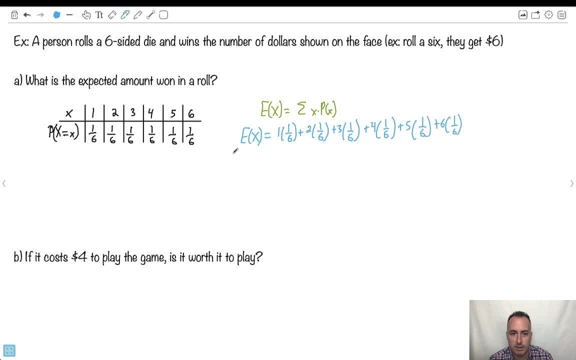 In this case, we have this All right Now. if I keep going, then what's the probability? Sorry, the expected value is one times one over six, which is one over six plus two over six, plus three over six. 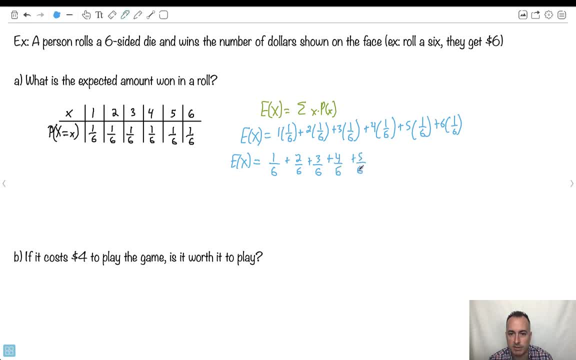 plus four over six, plus five over six, plus six over six. Then I can add them up: Well, they've got a common denominator. so that's kind of nice. So I can go six plus five plus one, for, Oh, actually you know what I'll do. 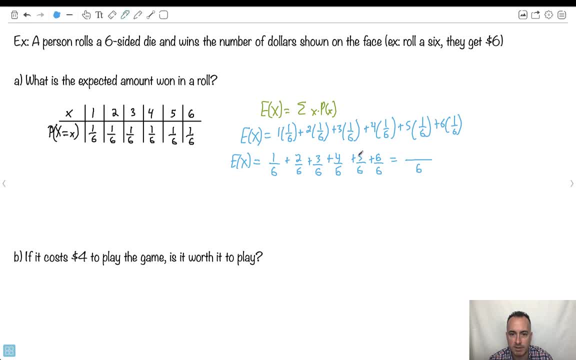 I'll do: four plus six is ten, Plus five is fifteen. That gives me eighteen, twenty, twenty-one. So I've got twenty-one over six. Now I can do it. This is the exact value, okay, So I'll say: 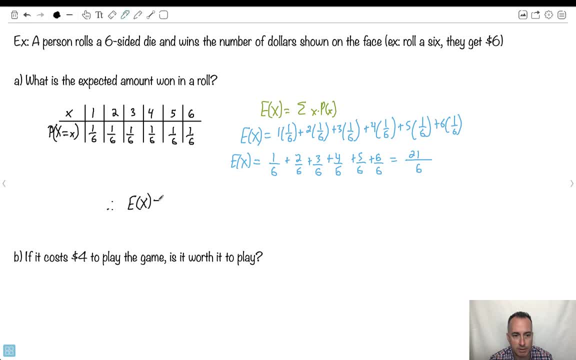 So the expected value is going to be twenty-one over six, Unless it divides by. Oh no, never mind, I can reduce it. actually It divides Twenty-one. can divide by three, It's seven, And six divides by three. 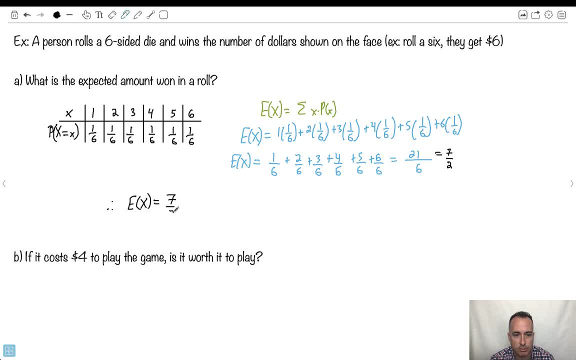 It's two, So it's actually going to be seven over two, which is going to be What's that? Three point five. If you want it on your calculator, you can do it that way. This is the answer. So you might wonder like: 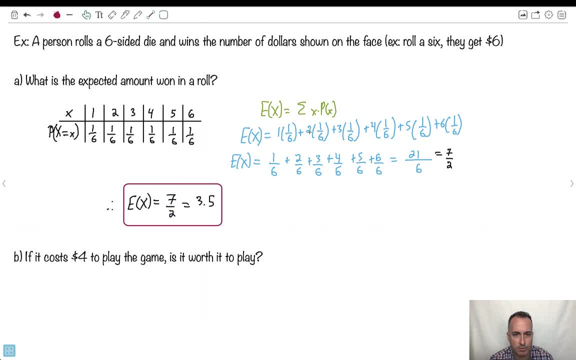 wait, aren't probabilities? Don't probabilities have to be less than one? Yeah, the probabilities do, But this isn't probability we're doing now. We're using probabilities. sure, There's probabilities within this, But the expected value? There's nothing that says expected value can't be greater than one. 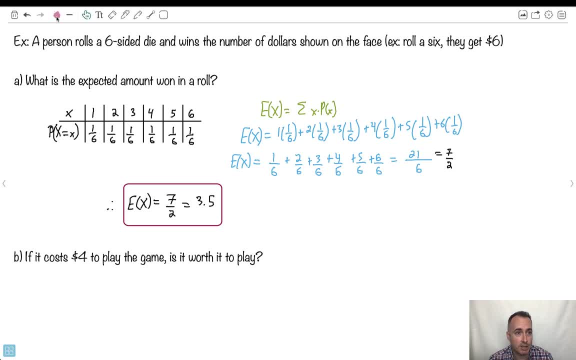 In fact, it often is. So what this really tells you is that you expect to win. This is maybe the conclusion, right? You expect to win about $3.50 each game. This is what you would be expected to win. 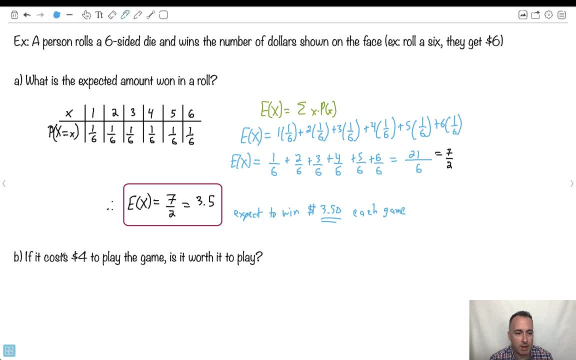 Okay, so that's how we could use this. Now, if it costs $4 to play the game, is it worth it to play? Well, no, Why not? It costs more. It costs more to play than your winnings, or at least your expected winnings. 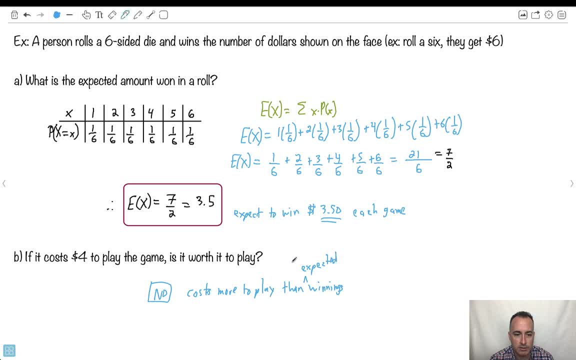 So this is. I think you could say that, So that's why you probably shouldn't play. By the way, this is how casinos work. They always make sure that they've calculated the expected earnings and make sure that they charge you more on average. 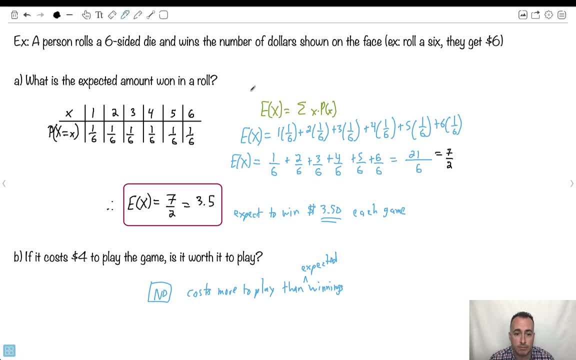 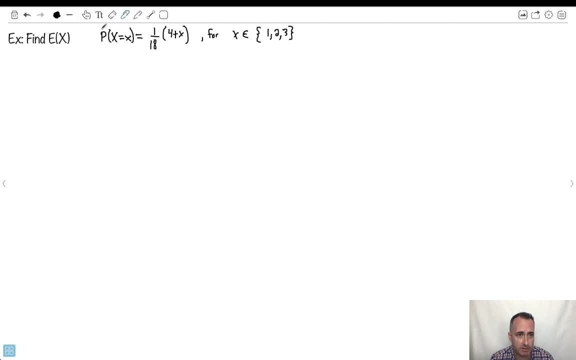 That's why casinos make money. So we can do another example. So here's another example. here We have the expected value We want to do. the expected value of this P of x equals x. So capital X equals lowercase x of 1 over 18, 4 plus x. 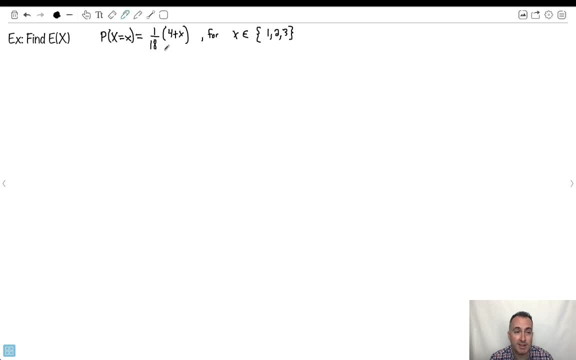 where x is an element of 1,, 2, and 3.. This looks complicated, sure, But let's just break it down here. Let's figure out what's the expected value. Well, it's equal to the sum of every x times every probability of getting that x. 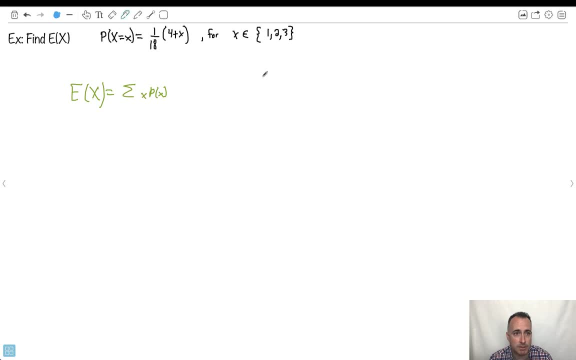 So all we have to do then is just make a table. Maybe I'll make a table now, Lowercase x, here We'll do So. if I get a 1,, I can get a 2, and I can get a 3.. 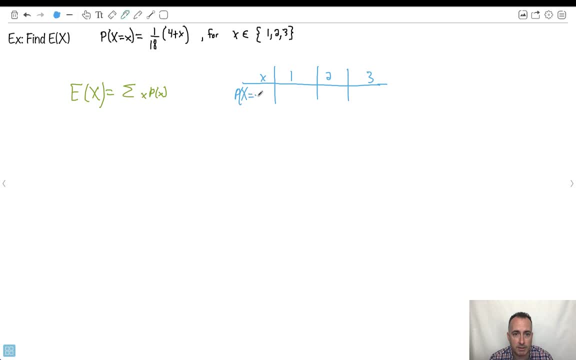 And I want the probability of that big X being little x here. What's the probability of getting a 1?? This is just a rule for the probabilities here, So watch If I get a 1 here. 1 plus 4 is 5.. 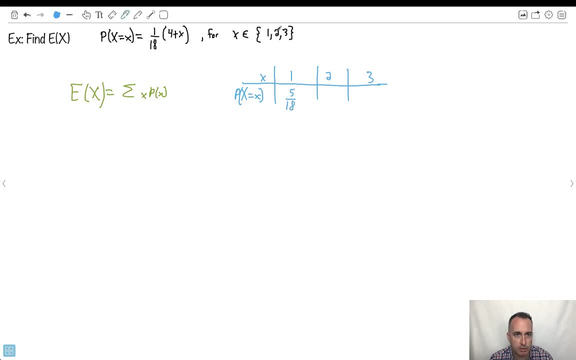 So that's 5 over 18. How about 2 here? 2 plus 4 is 6. So 6 over 18.. 3. So 4 plus 3 is 7. 7 over 18.. 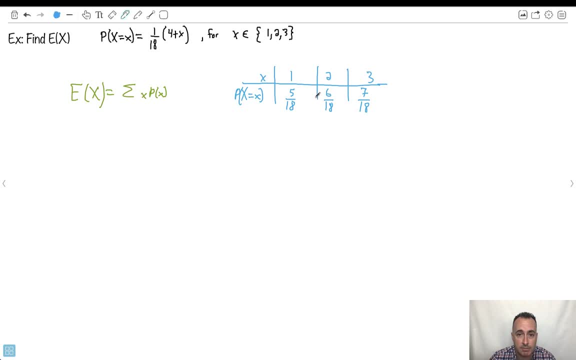 Now, if it's a real probability distribution function, these had better add up to 1.. Let's see: 5 plus 6 is 11.. 11 plus 7 is 18.. Good, 18 over 18.. So this works. 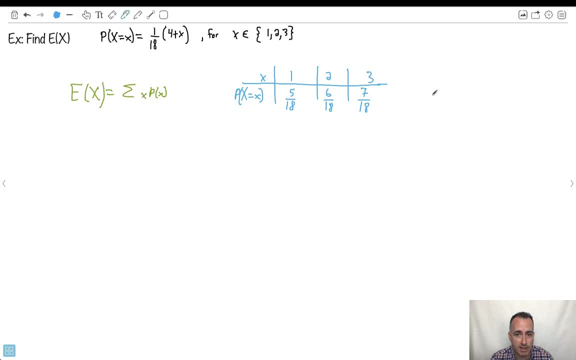 This will be a real thing. Remember, the probabilities always have to add up. Remember, the sum of all the probabilities has got to be 1.. So this seems to work. So now we can go ahead and calculate the expected value. 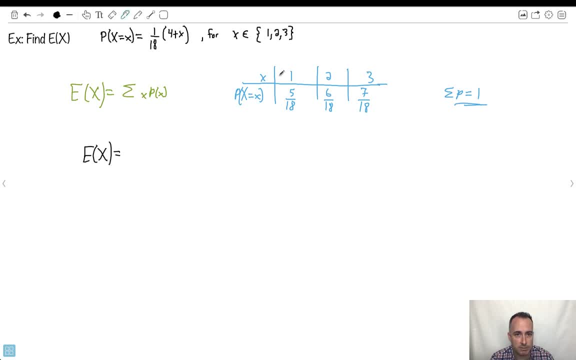 So the expected value will be: Let's see, I just multiply every x times its p of x, So I go 1 times 5 over 18 plus 2 times 6 over 18 plus 3 times 7 over 18.. 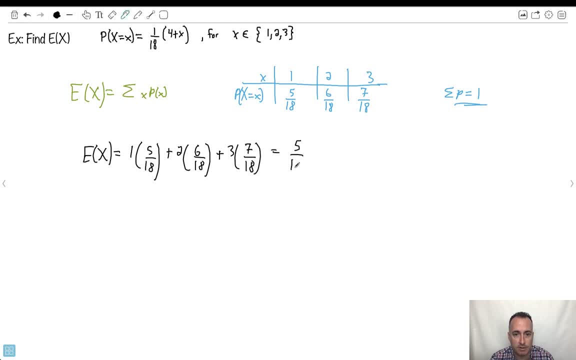 All right. So what do I do here? 1 times 5 is 5 over 18.. 2 times 6 is 12 over 18.. And 3 times 7 is 21 over 18.. All right? 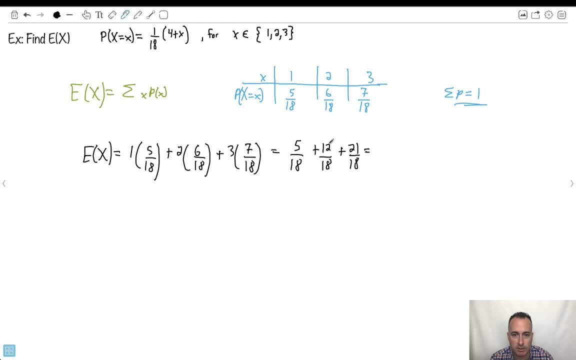 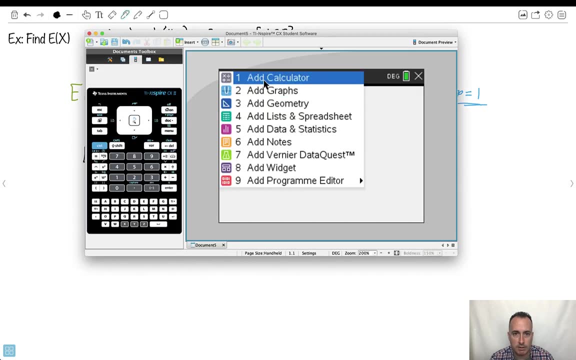 So that would be. Let's see, This is 21 plus 12.. So that's 33.. That'll be 38 over 18.. Do that on my trusty old calculator here. What's 38 divided by 18?? 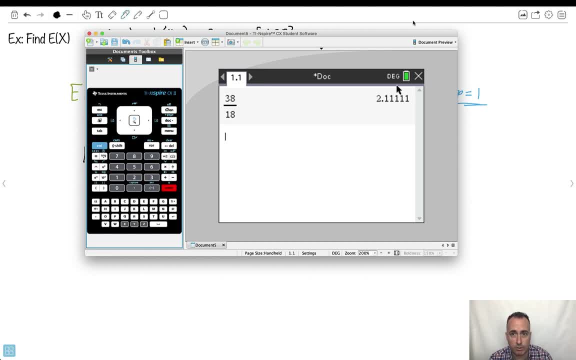 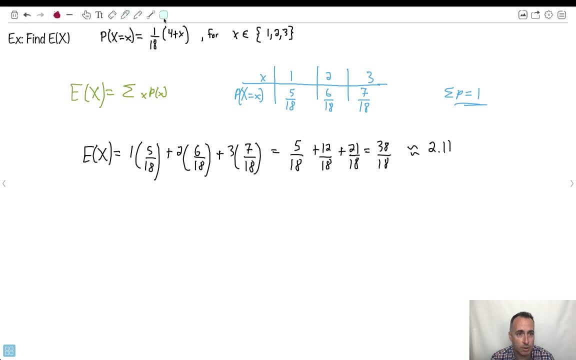 Give me the answer. It's 2.11, roughly, So approximately 2.11.. That's my expected value. I'm done So. although this stuff looks really complicated, there's nothing to it, right? All you have to do is just look at this equation here. 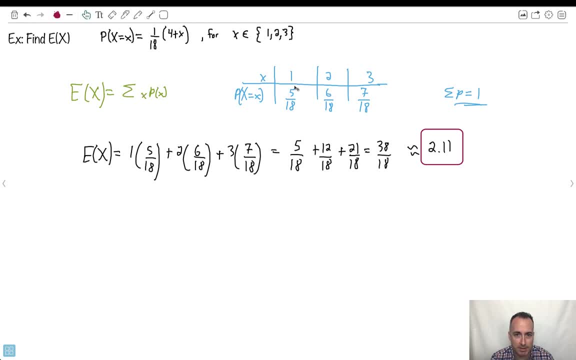 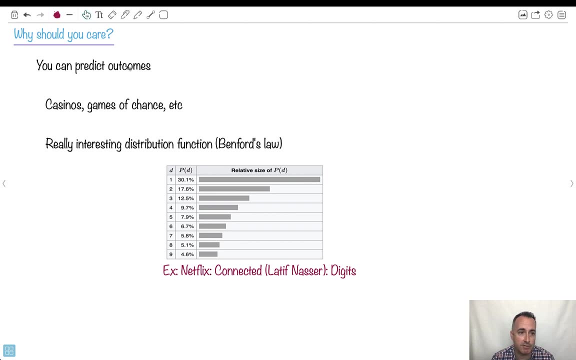 Take every x, Multiply it by its probability, Add up the next x and its probability, Add up the next one. Just keep going. That's your expected value. Now why should you care? I mean, this is useful for predicting. 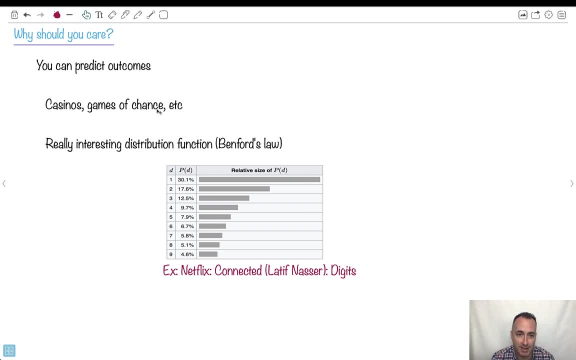 Casinos, game of chance- all that stuff works this way. I thought a really interesting one is: sometimes things break from what's expected. There's something called Benford's Law. I can tell you this When I first learned about this- I'm not kidding when I say I never saw the world the same again. 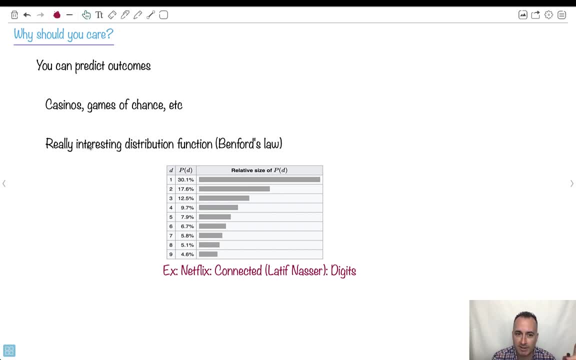 This is true. There's this weird thing. See, we would expect. This is really weird. It turns out you would expect if you saw a bunch of random numbers. Let's just say I gave you, like here's a population of all the towns, of all the major. 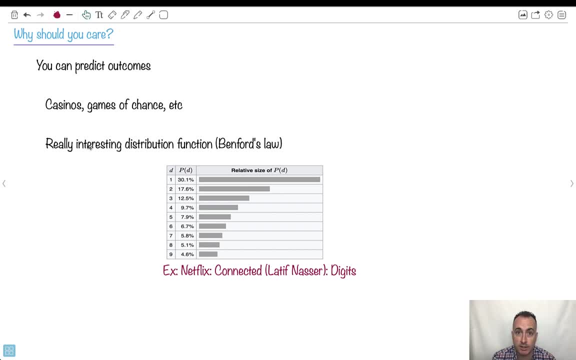 cities in your country. Let's say the population of the major cities in your country. What you would do is no matter what the population is, whether it's a million or 100,000 or 50,000, whatever, or 1,000 or 200, whatever. 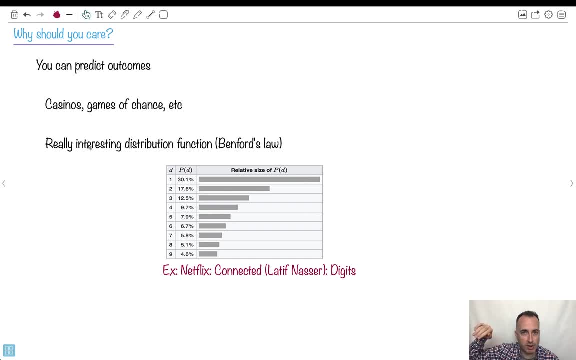 This really weird thing is that if you take all the digits to the right and you remove them and you just keep the leading number, the first number you see, you would expect those to be pretty random, wouldn't you? You'd expect them to be like 1s, 2s, 3s, 4s, 5s, 6s, 7s, 8s and 9s should be equally likely. 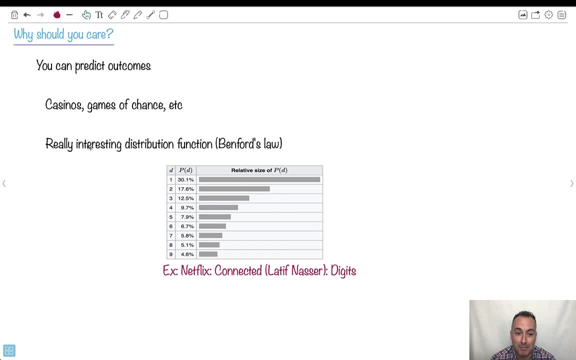 You would expect that, wouldn't you? Benford's Law shows that. nope, we have this probability distribution function that actually does not match what's expected. It turns out the preponderance, like the number of times you get a leading 1, is actually 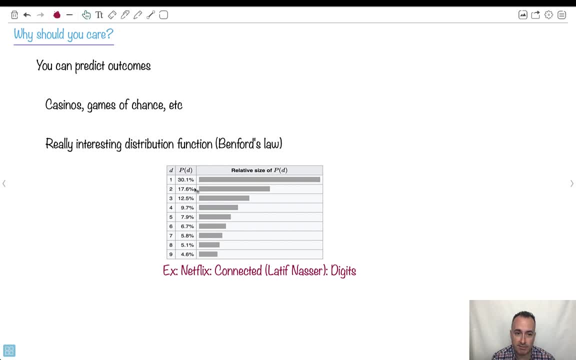 30% for some weird reason, And a 2 is actually 17% And a 3 is like this. This actually follows a distribution function. It actually follows a function that goes like: what would it be here? I think it's the probability of getting D.